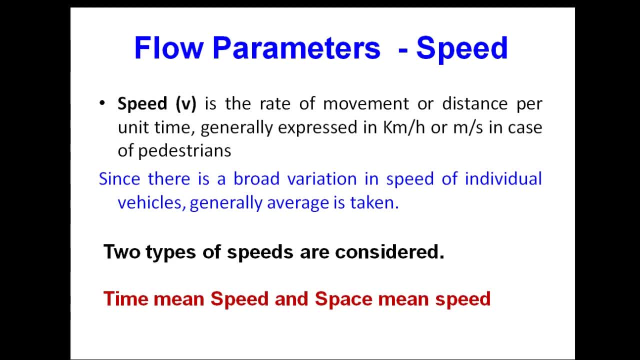 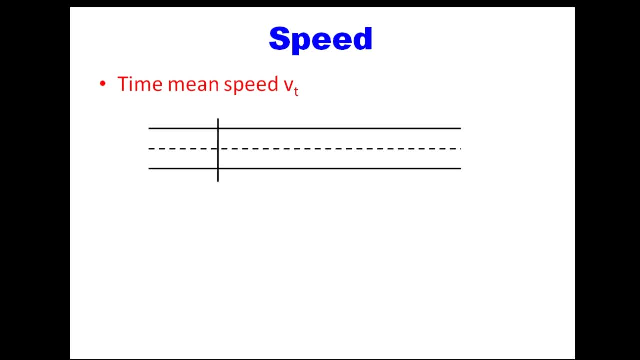 called time mean speed and another is called space mean speed. So time mean speed is like this: that if you take a section of the road and you stand on a reference line here, when they cross this line you find out the speed of individual vehicle, let us say n vehicles. 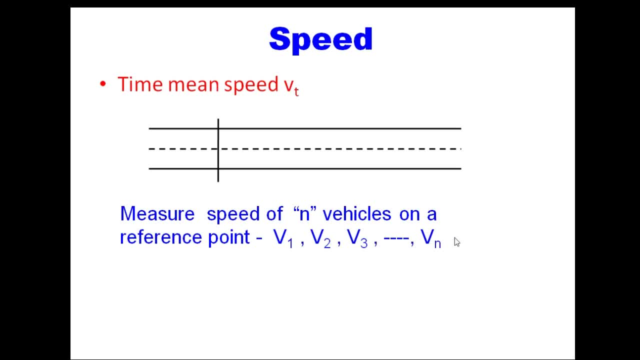 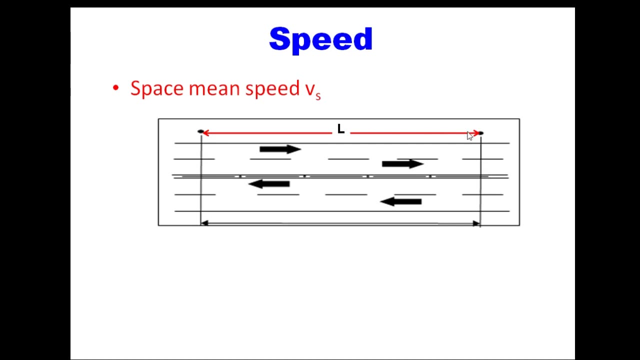 v1, v2, v3 and so on, vn. then arithmetic average of these speeds is called the time mean speed, simple. but when you take the same highway and on the on this highway you consider a section of length l and then try to find out how much time individual vehicle will take to cover this length. 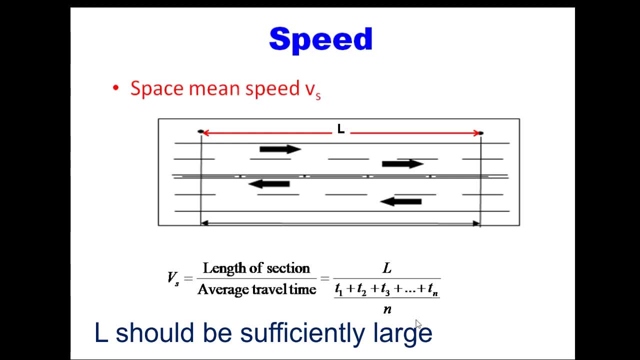 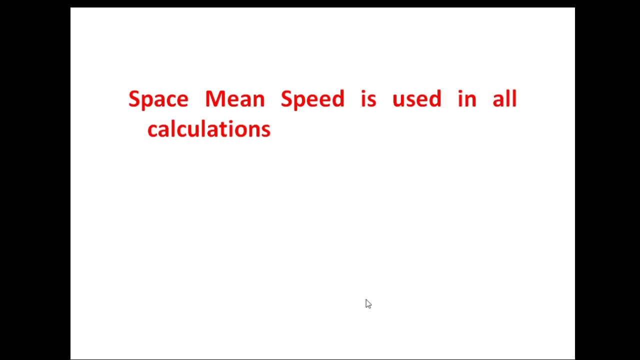 of section. then this: t1, t2, t3 are the time taken by n vehicles to traverse this length. l then space: mean speed is defined as the length of the section divided by average time taken by these vehicles. so speed means speed is used in all calculations in traffic engineering. 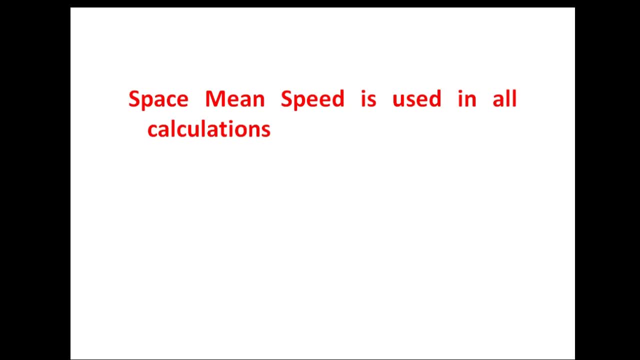 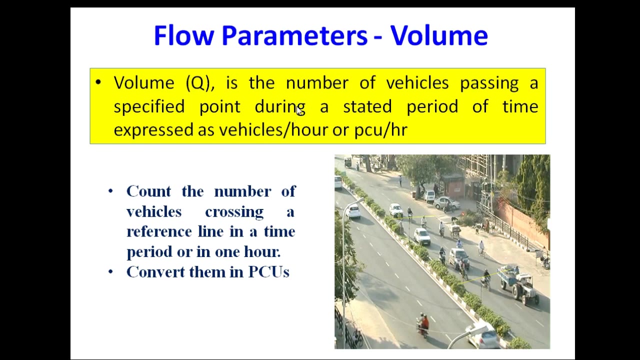 now you can calculate space mean speed from time mean speed also, and time mean speed from space mean speed data also, and there is a mathematical correlation between these two. the next parameter is the volume. traffic volume is defined as the number of vehicle passing a specified point during. 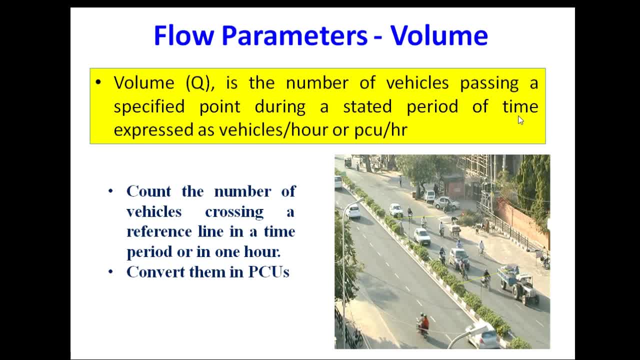 a period of time, and time generally is taken as one hour and therefore the traffic volume is expressed as vehicles per hour or pcu passenger car unit per hour. so this is the highway and if this is a reference line, so if you stand here and count the number of vehicle passing this reference, 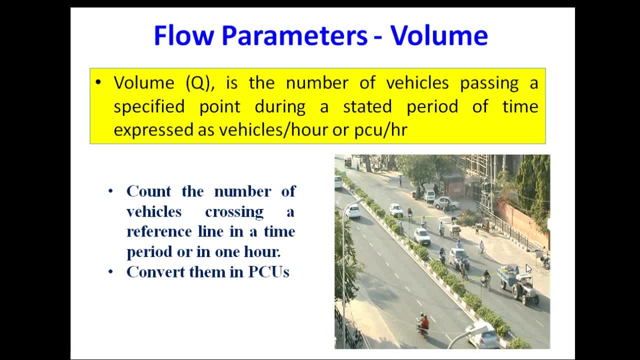 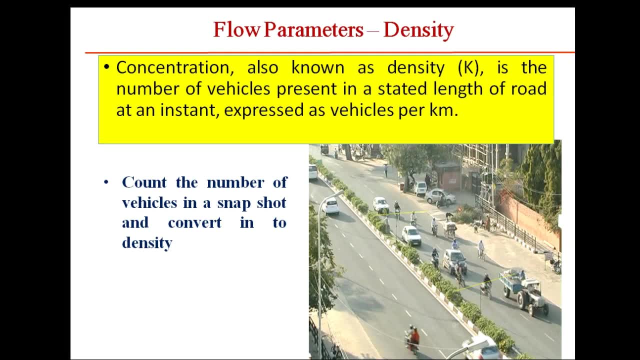 line one hour. that is traffic volume. similarly, the third parameter is the density concentration: number of vehicles present in a stated length of the road at any point of time, and length is one kilometer. so if you take a aerial shot, a photograph of a highway, and let us say you mark some length on this highway, ideally should be one kilometer. 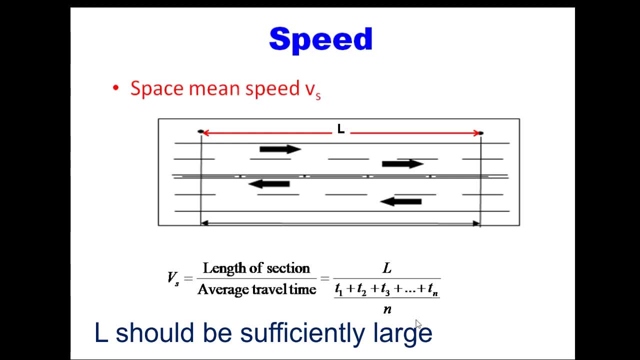 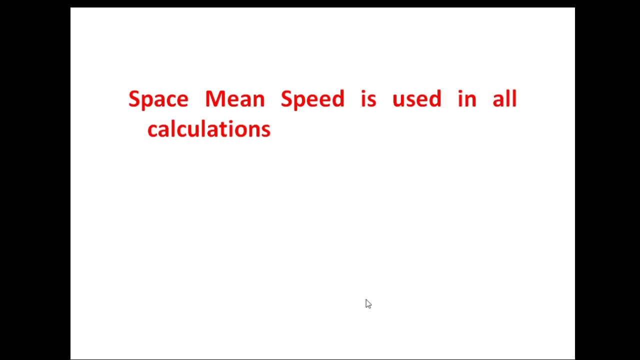 of section. then this: t1, t2, t3 are the time taken by n vehicles to traverse this length. l then space: mean speed is defined as the length of the section divided by average time taken by these vehicles. so speed means speed is used in all calculations in traffic engineering. 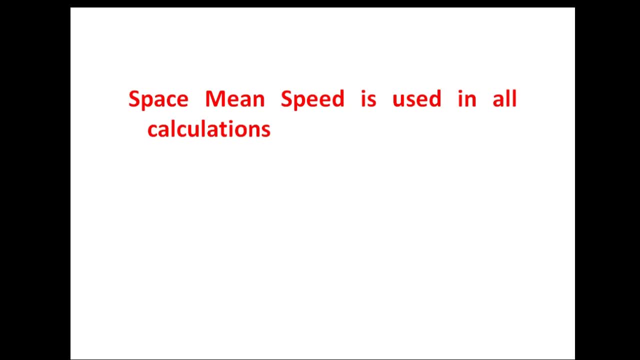 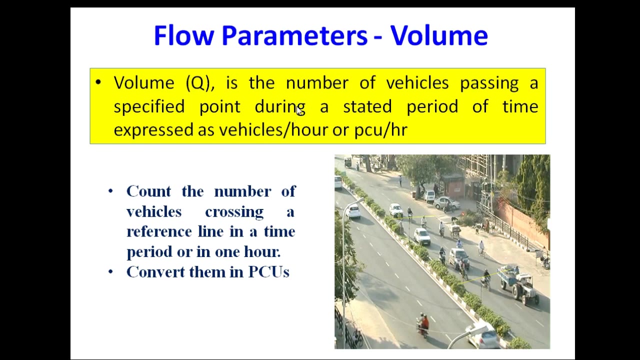 now you can calculate space mean speed from time mean speed also, and time mean speed from space mean speed data also, and there is a mathematical correlation between these two. the next parameter is the volume. traffic volume is defined as the number of vehicle passing a specified point during. 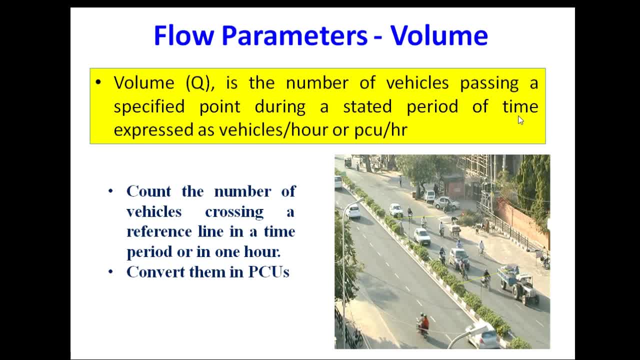 a period of time, and time generally is taken as one hour and therefore the traffic volume is expressed as vehicles per hour or pcu passenger car unit per hour. so this is the highway and if this is a reference line, so if you stand here and count the number of vehicle passing this reference, 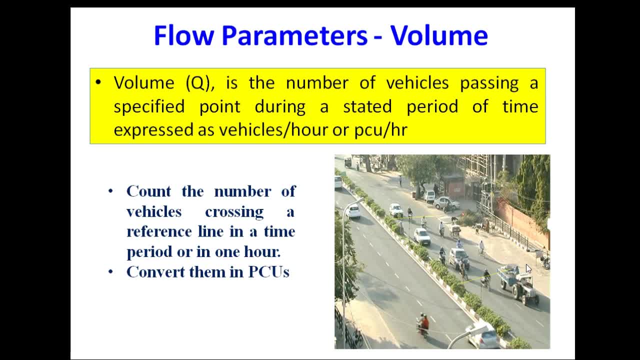 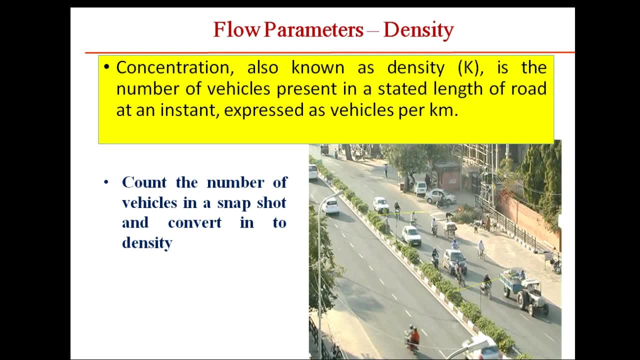 line one hour. that is traffic volume. similarly, the third parameter is the density concentration: number of vehicles present in a stated length of the road. so if you take a aerial shot at any point of time and length is one kilometer. so if you take a aerial shot, a photograph of a highway, let us say you mark some length on this highway, ideally it. 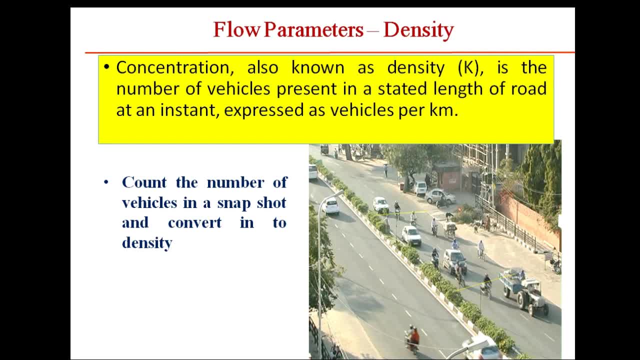 should be one kilometer, but that one kilometer can only be covered through drones. but if you are taking photograph using your camera, you define certain length, let us say 200 meter. Then in this snapshot you count the number of vehicles which are within this snapshot. 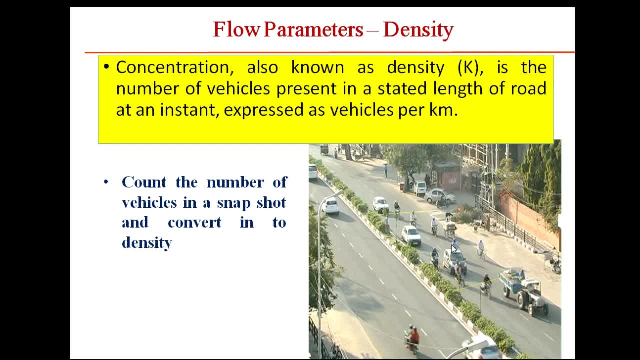 of 200 meter and then extrapolate this number to 1 kilometer. that is the density. Density is in vehicles per kilometer. If there are more than one lane in one direction, we say vehicles per kilometer per lane. Now, these three parameters- speed, density and flow, they are macro parameter. 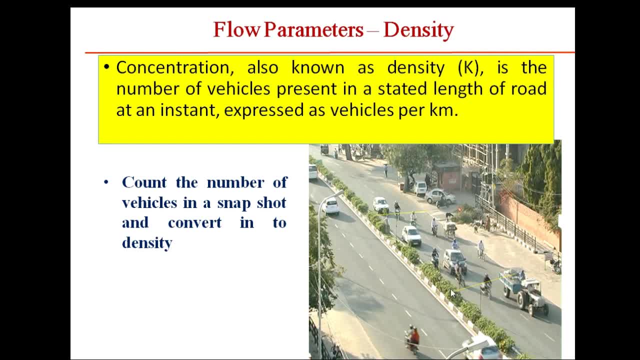 but that one kilometer can only be covered through drones. but if you are taking photograph using your camera, you define certain length, let us say 200 meter, and then in this snapshot you have the length. that is the distance, the distance from the road to the highway, and you have the length of the road. 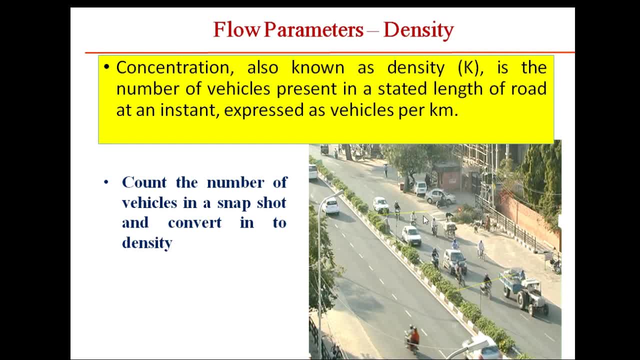 you count the number of vehicles which are within this snapshot of 200 meter and then extrapolate this number to one kilometer. that is the density. density is in vehicles per kilometer. if there are more than one lane in one direction, we say vehicles per kilometer per lane. 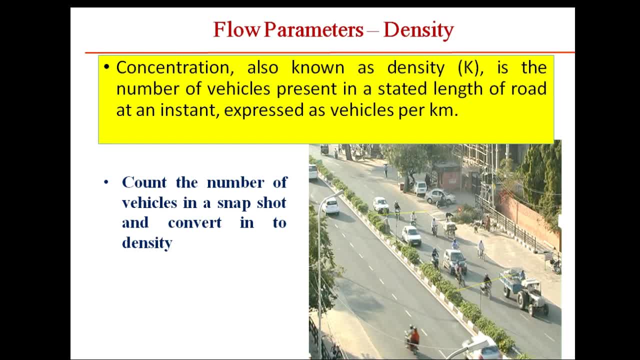 now these three parameters: speed, density and flow. they are macro parameter. macro means basically that you are taking an average of different way kills. they are not considered in divisible vehicle. when we define space mean speed, it is placed in the speed of the entire stream: traffic volume in one hour or density in one kilometer. in addition to these three, 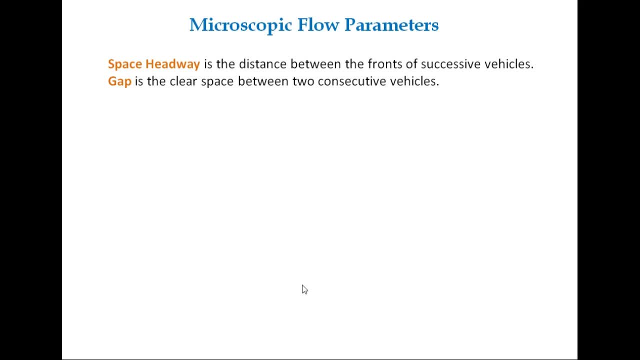 parameters. there are two microscopy flow parameter was headway and gap. they can also be measured either in meter or in second and accordingly we say space headway, gap, or time headway or time gap. space headway is the distance between the fronts of two successive vehicles, whereas gap is the clear space between two consecutive vehicles. so if 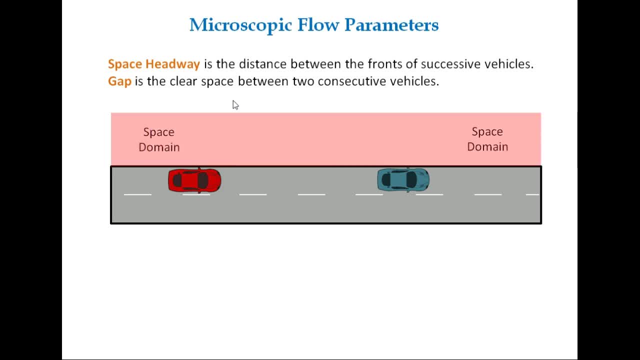 you take section of the road and this is the space domain, then when you measure the distance between front of the vehicles, front of two successive vehicle, then this becomes space headway and when you measure the clear distance between the two, then this is the gap. similarly, time headway is the time. 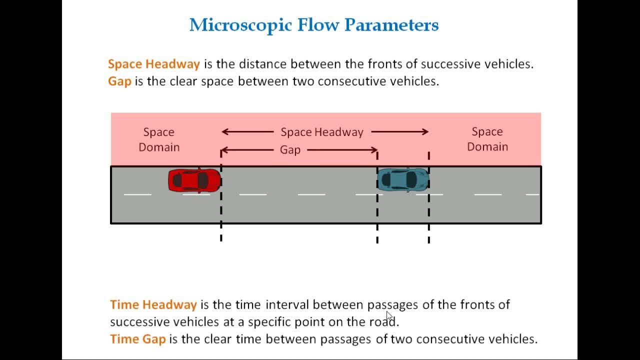 interval between passage of the front of successive vehicles at a specified point of on the road and same same highway. if you consider time diagonal in below this line, then time headway is the time difference between the passing of front of the two successive vehicles and time gap is the clear distance between the two vehicles. you can. 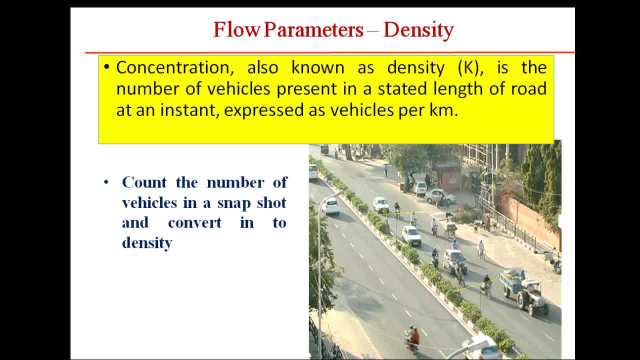 Macro means basically that you are taking average of different vehicles. They are not considered individual vehicles. When we define space mean speed, it is the space mean speed of the entire stream, Traffic volume in one hour or density in one kilometer. In addition to these three parameters, there are two parameters. 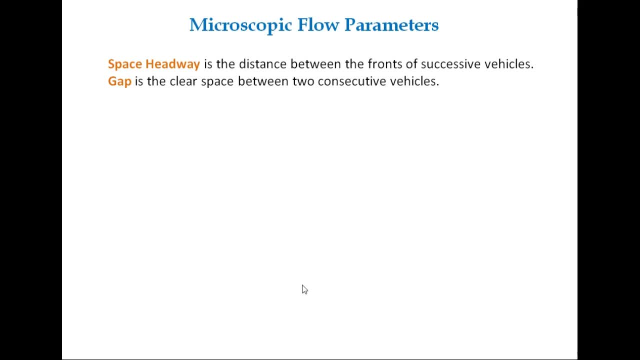 There are two microscopic flow parameters also: headway and gap. They can also be measured either in meter or in second And accordingly we say space headway gap or time headway or time gap. Space headway is the distance between the fronts of two successive vehicles, whereas 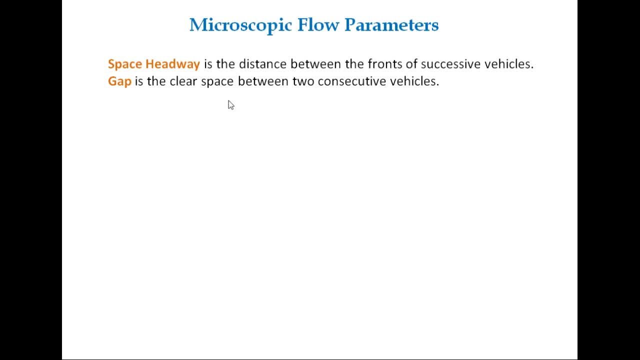 gap is the clear space between two consecutive vehicles. So if you take a section of the road And this section of the road is the distance between the fronts of two consecutive vehicles, This is the space domain- Then when you measure the distance between front of the vehicles, front of two successive, 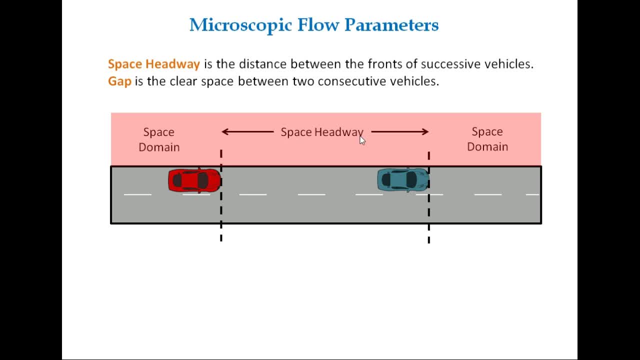 vehicles, then this becomes space headway, And when you measure the clear distance between the two, then this is the gap. Similarly, time headway is the time interval between passage of the front of successive vehicles at a specified point on the road. 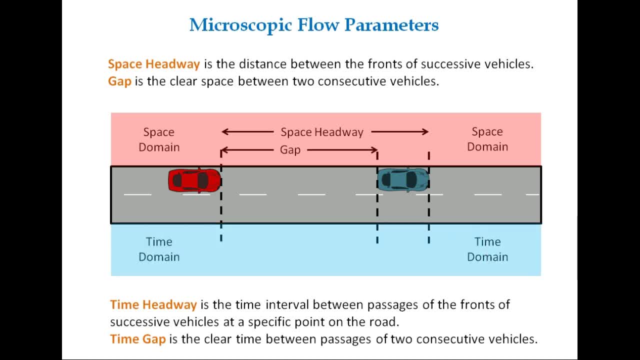 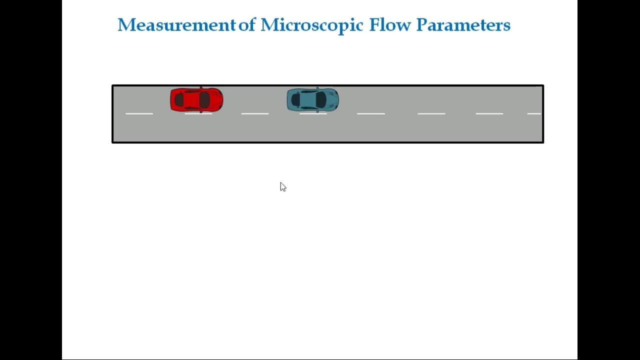 Same same highway. If you consider time domain below this line, then time headway is the time difference between the passing of front of the two successive vehicles and time gap is the clear distance between the two vehicles. You can understand it like this also, that on a section of the road, if this is the reference, 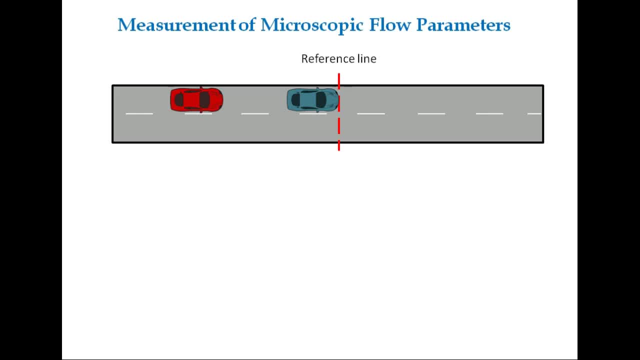 line. If you take the time of arrival of different vehicles on this reference line and you start counting the time- t1 when the front bumper of the vehicle is on the reference line, then t2 is the time when the front bumper of second consecutive vehicle. consecutive next vehicle. 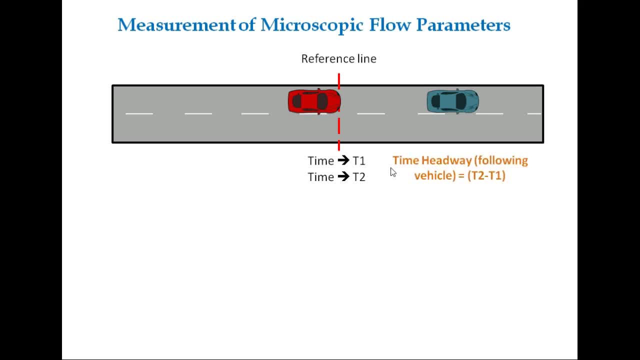 is on the reference line, then t2 minus t1 will be the time headway. And if you know the speed of this following vehicle, you can find out the space interval, space headway, by multiplying this time headway by the speed of the following vehicle. 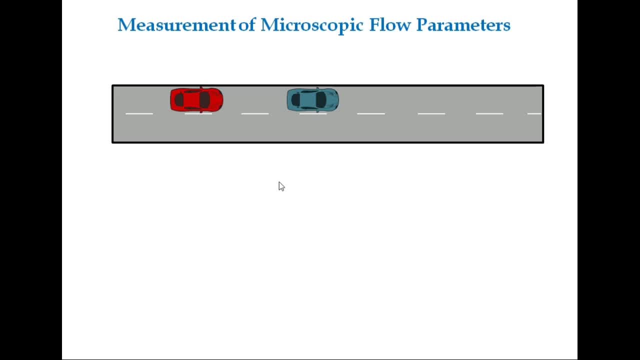 understand it like this also, that on a section of the road, if this is the reference line, note down the time of arrival of different vehicles on this reference line and you start counting the time. t1 when the front bumper of the vehicle is on the reference line, then t2 is the. 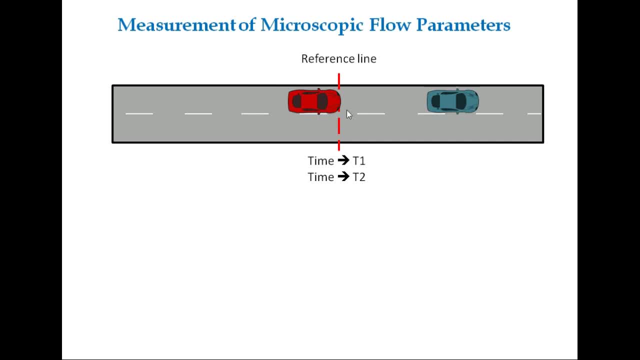 time when the front bumper of second consecutive vehicle, consecutive next vehicle is on the reference line, then t2 minus t1 will be the time headway and if you know the speed of this following vehicle, you can find out the space headway by multiplying this time headway by the speed of the following vehicle. 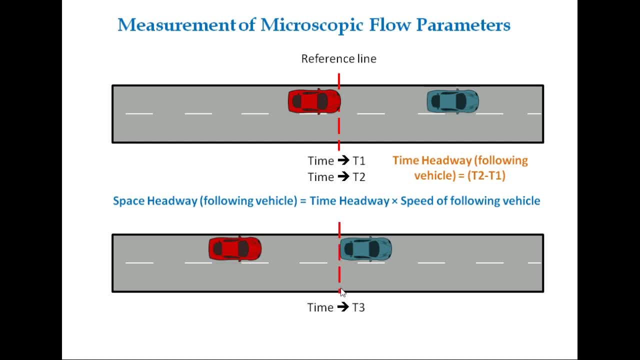 Similarly, if you consider the reference line starting the back of the first vehicle and then you consider the time t4, when the front bumper of the next vehicle is on the reference line, then t4 minus t3 is the time gap, and again this time gap multiplied by the speed of following. 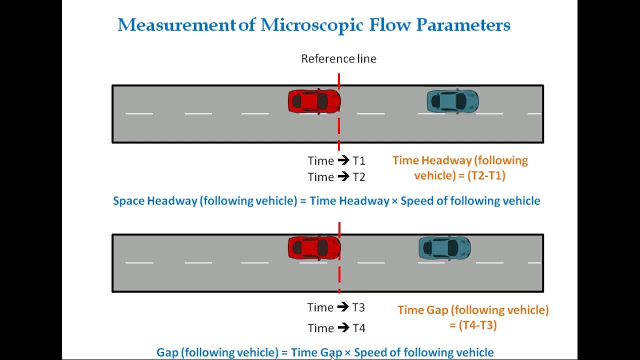 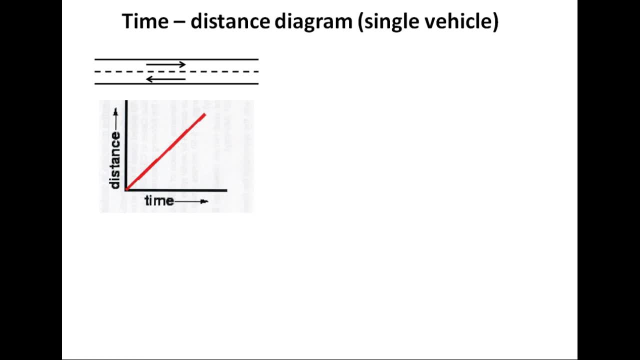 vehicle will give you the space or the clear gap. this is the time-distance diagram of a single vehicle which is moving at a constant speed. So a vehicle moving at constant speed. the distance will continuously increase with time, and slope of this line will give you the speed of the vehicle. 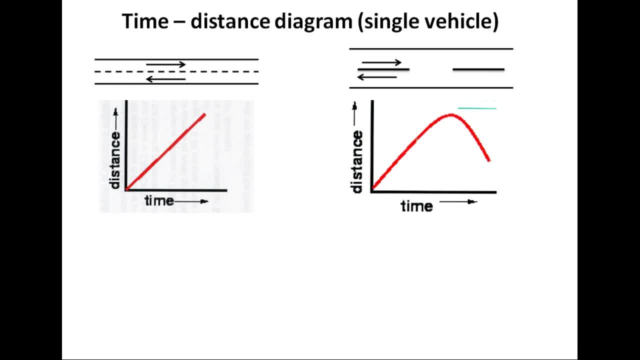 This is the vehicle which is moving at some constant speed, that is, start decelerating and then move in reverse direction. Now this may be the case when a vehicle here coming from this direction, it takes a? u turn at the median. Now the third case is when you have a vehicle approaching a signal control intersection. 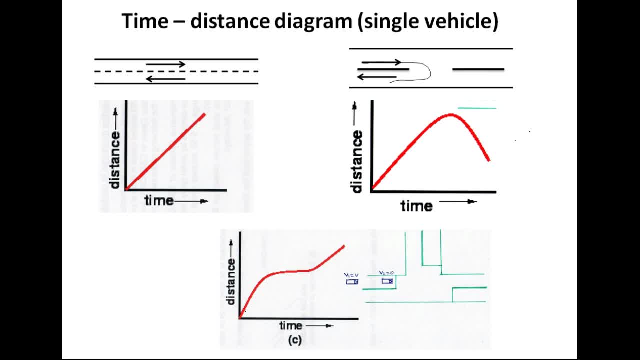 When a vehicle approaching signal control intersection will be moving in the approach at a constant speed. when he sees the traffic light is red, start decelerating, come to stop here, the stop line for some time, until the until the green time appears, and then it starts decelerating. 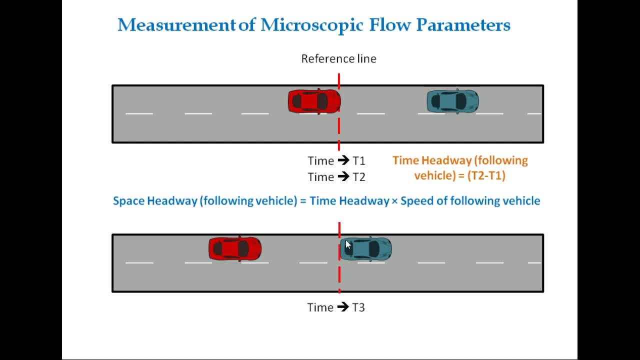 Similarly, if you consider the reference line starting the back of the first vehicle and then you consider the time t4, when the front bumper of the next vehicle is on the reference line, then t4 minus t3 is the time gap, And again this time gap multiplied by the speed of following vehicle. 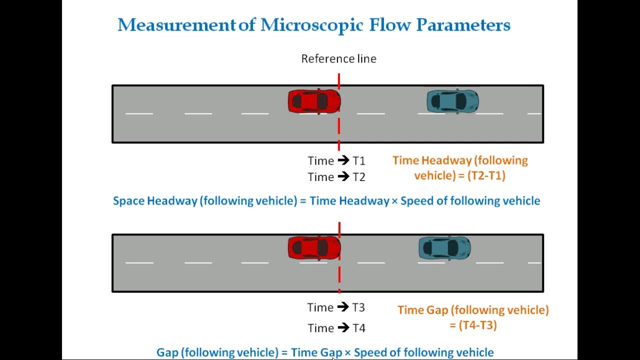 Similarly, if you consider the reference line starting the back of the first vehicle and then you consider the time headway, by multiplying this time headway by the speed of following vehicle, you can find that t3 minus t4 will be the time headway where the second vehicle. 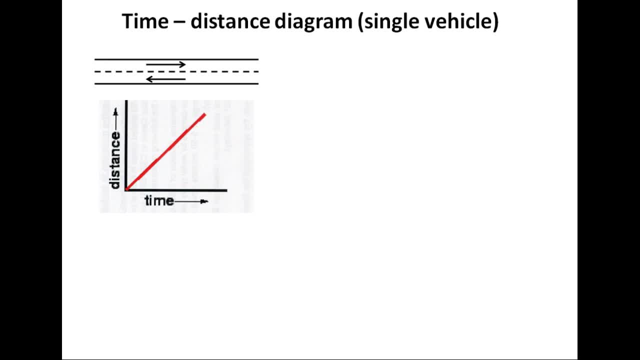 and HEL drives pass each other. This is the time distance diagram of a single vehicle which is moving at a constant speed. So a vehicle is moving at a constant speed. The distance will continuously increase with the time, And slope of this line will give you the speed of the vehicle. 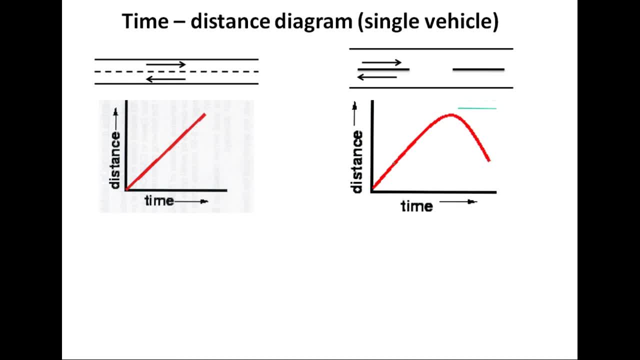 This is the vehicle which is moving at the same speed as the vehicle starting it. This is the vehicle which is moving at a constant speed, moving at some constant speed, that is, start decelerating and then move in reverse direction. now this may be the case when a vehicle here coming from. 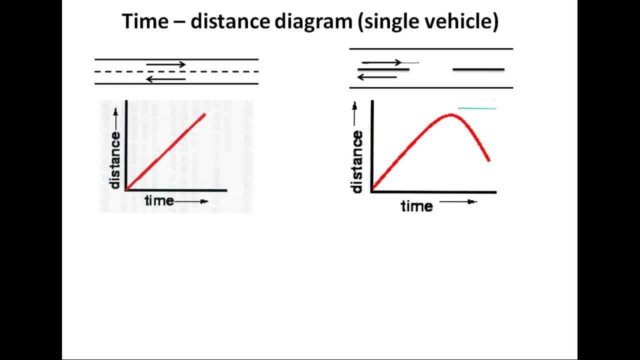 this direction. it takes a u-turn at the median. now the third case is when you have a vehicle approaching a signal control intersection. my vehicle approaching signal to control intersection will be moving in the approach at a constant speed when he sees the traffic light is red start. 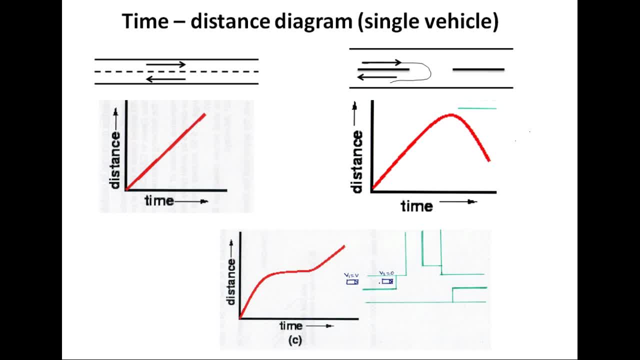 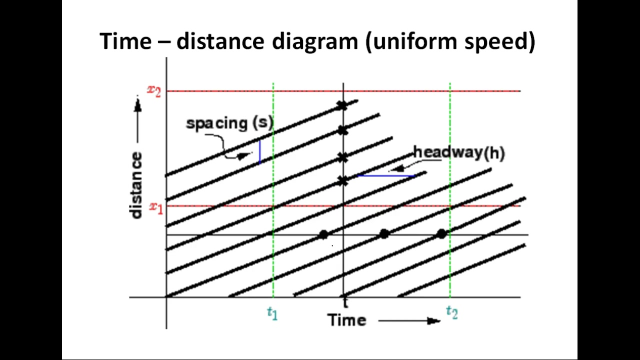 decelerating, come to stop here, the stop line for some time, until the, until the green time appears, and then it starts accelerating and then reach to the straight line again at a normal speed. now, when you have a series of vehicles on a road and all are moving at a constant speed, then these are the lines, these are the. 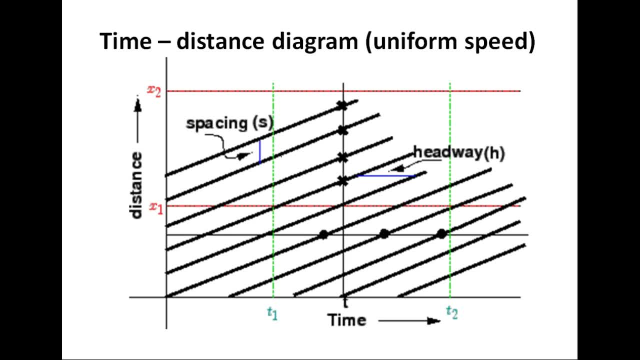 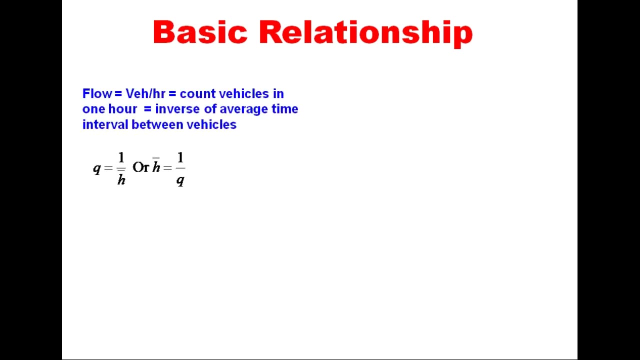 trajectory of different vehicles. they will parallel. these lines will be parallel and the vertical distance between any two line will give you the spacing between the vehicles and the horizontal distance between the two line will give you the time head Estimated. I Grande what we have understood so far. I defined the flow or volume as the vehicle per. 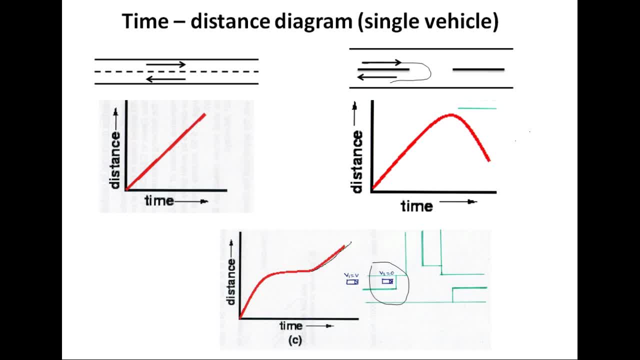 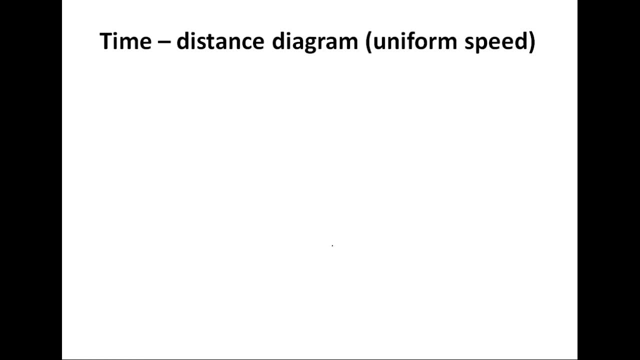 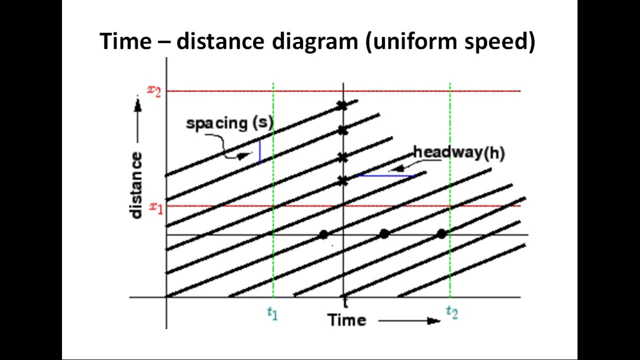 Accelerating and then reach to the straight line again at a normal speed. When you have a series of vehicles on a road and all are moving at a constant speed, then these are the lines, these are the trajectory of different vehicles. they will be parallel. these lines will be parallel and the vertical distance between any two line will give you 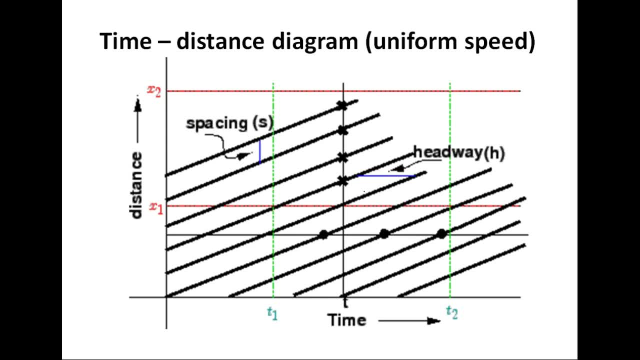 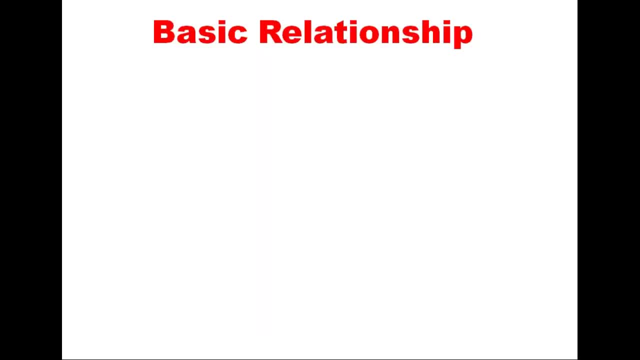 the spacing between the vehicles and the horizontal distance between the two line will give you the time headway, What we have understood so far. I defined the flow or volume as the vehicle per hour, which is the count in one hour. count of vehicles in one hour. 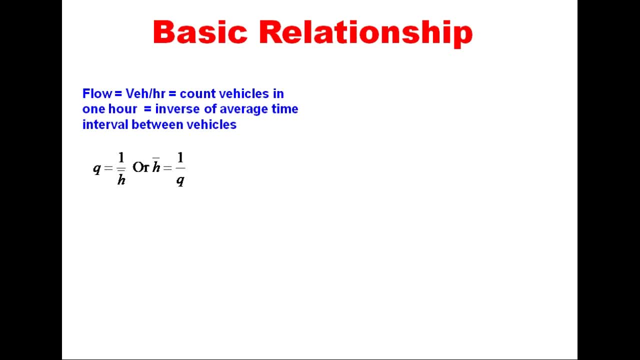 So if you stand on a highway and let us say, you count the number of vehicles in one hour and you find that There There are one thousand eight hundred vehicles, That means on an average every two second there is a vehicle passing the reference line. 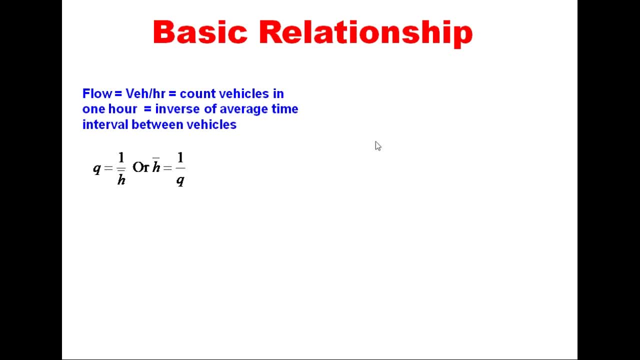 Now this two second is the time interval between the vehicle. so you can say time headway, So Q will be inverse of this time headway. or you can say the average time headway is inverse of flow. Similarly, density: we defined the number of vehicles in one kilometer length of the road. 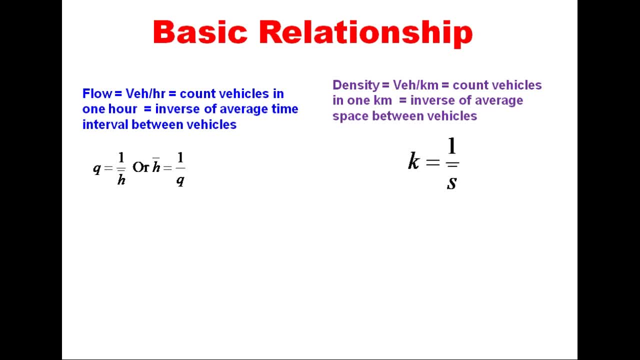 So if you take a snapshot of one kilometer and you find there are hundred vehicles in the snapshot, that means on an average there is ten meter distance between the two vehicles. So space headway, the density is the inverse of space headway, or you can say space headway. 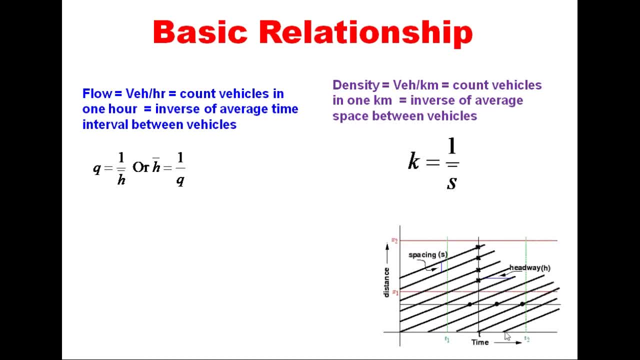 is inverse of density and you remember this graph, the trajectory of different vehicles moving at the constant speed. And I told you that the vertical distance is the spacing and horizontal distance is the time headway and the slope of each line will be the space divided by time. 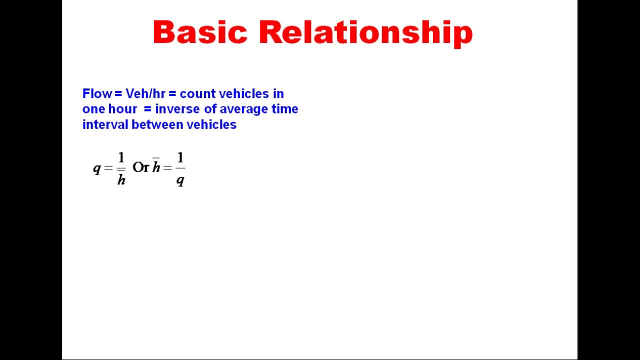 hour, which is the count in one hour, count of vehicles in one hour. so if you stand on a highway and it is a, you count the number of muchísimo and you find that there are 1500 vehicles. 'tagh, lemme go ahead and try fx this thing. 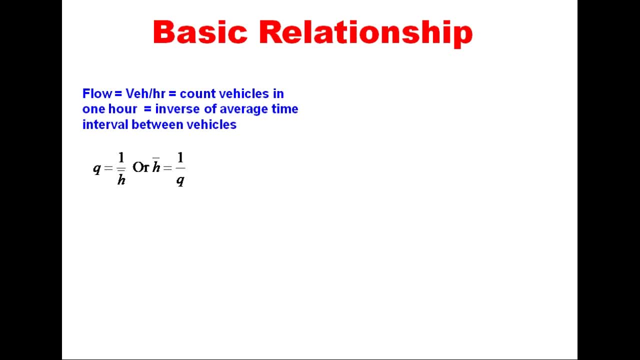 and you will. this work like that. That means on an average, every 2 seconds there is a vehicle passing the reference line. Now this 2 seconds is the time interval between the vehicles. or you can say time headway, So Q will be inverse of this time headway. or you can say the average time headway is inverse of flow. 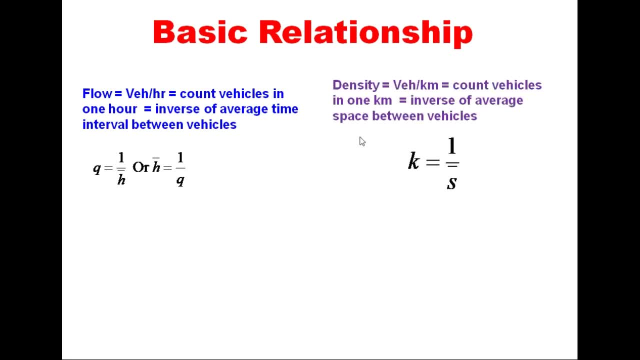 Similarly, density will be defined as the number of vehicles in 1 km length of the road. So if you take a snapshot of 1 km and you find there are 100 vehicles in the snapshot, that means on an average there is 10 meter distance between the 2 vehicles. 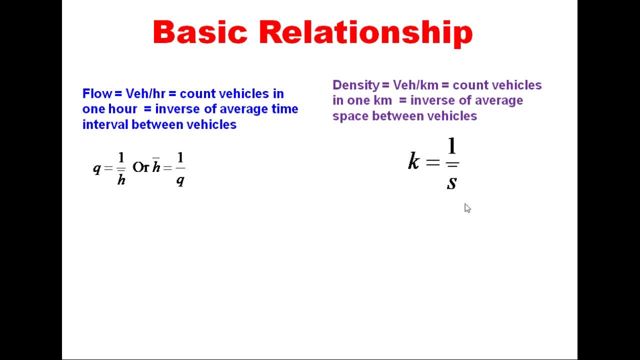 So space headway, the density is the inverse of space headway. or you can say space headway is inverse of density. And you remember this graph, the trajectory of different vehicles moving at the constant speed. And I told you that, the trajectory of different vehicles moving at the constant speed, 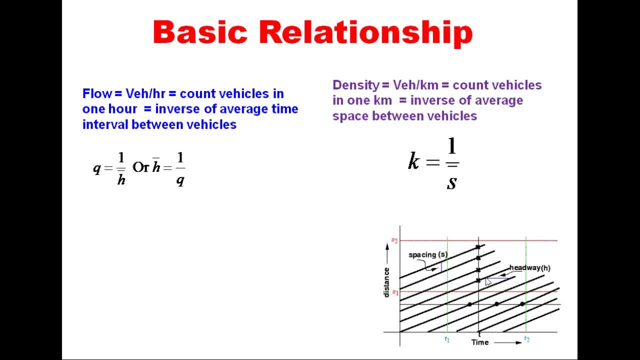 And I told you that the vertical distance is the spacing and horizontal distance is the time headway And the slope of each line will be the space divided by time. So speed will be space headway divided by time headway, Space, headway. you can write S or S bar. 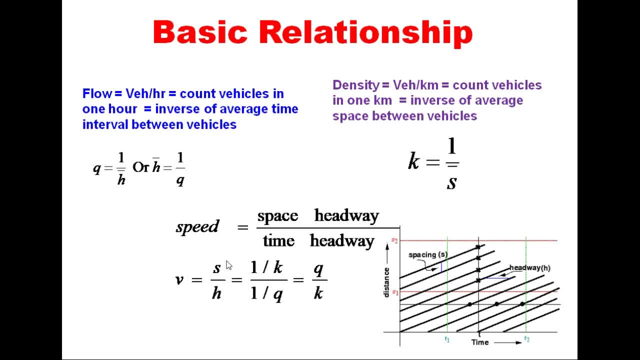 And time headway, H or H bar. S is 1 upon K from this equation And H is 1 upon K. So you can substitute these two values of S and H And that becomes Q upon K. So this gives you Q is equal to K into V. 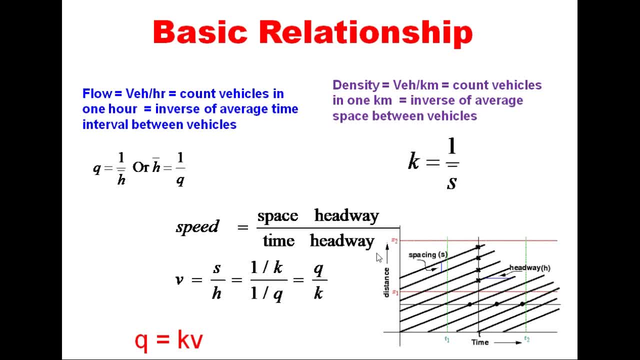 So that is how this correlation is derived. You can write your suggestions in the comment box. Thank you very much.